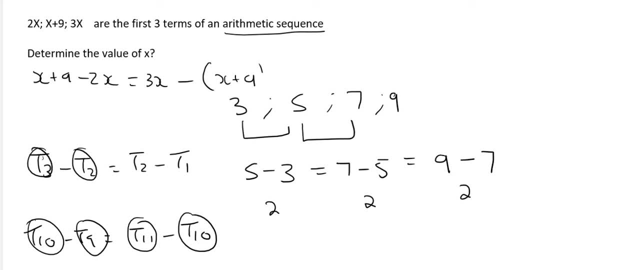 but now, because that x plus 9 is two terms, you would want to put it in a bracket like that and then you can solve, You see. so what we're doing here is we're manipulating the fact that the differences in an arithmetic pattern have to stay the same so we can form a relationship like that. 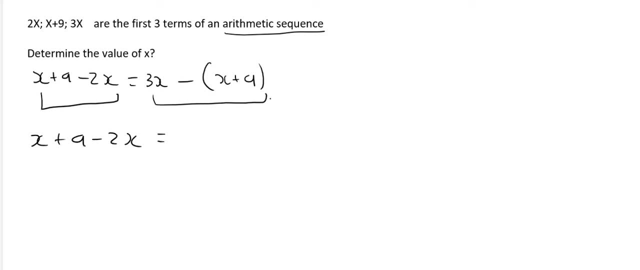 So what we have is x plus 9 minus 2x equals to 3x minus x minus 9, and now it's just a matter of solving for x. So on the left-hand side and on the right-hand side, we have that. then I'm going to. 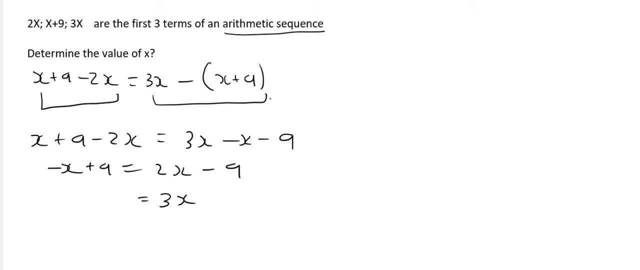 take all the x's to the right and then bring all the numbers over, and so what we find is that x is equal to 6.. So if you then wanted to carry on with the sequence, if there were other questions, you could fill in the actual values. So 2 times 6 is 12.. So you could fill in the actual values. so 2 times 6 is 12.. So if you then wanted to carry on with the sequence, if there were other questions, you could fill in the actual values. so 2 times 6 is 12.. 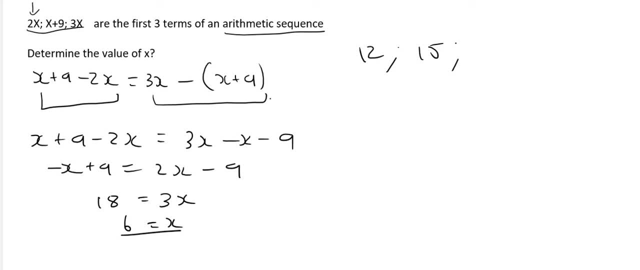 6 plus 9 is 15, and 3 times 6 is 18, and so this is the original pattern and then you could use that. if there were other questions, here's another one that we can practice. so we know that when it's arithmetic we can take the second term minus the first term and remember when you're minusing. 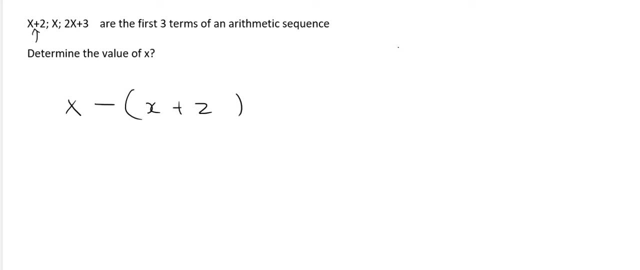 something with two terms, or two or more, two or more. you want to use a bracket, then you're going to make that equal to 2x plus 3, which is this term over here, minus the middle term, which is x, and you can put that in a bracket if you want, but there it's not going to make much of a difference. 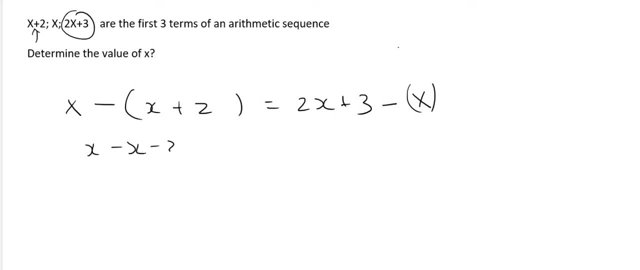 now what we do is we just solve so it becomes x minus x minus 2 equals to 2x plus 3 minus x. these x's cancel and so minus 2 is equal to x plus 3, because this 2x minus that x is just x. 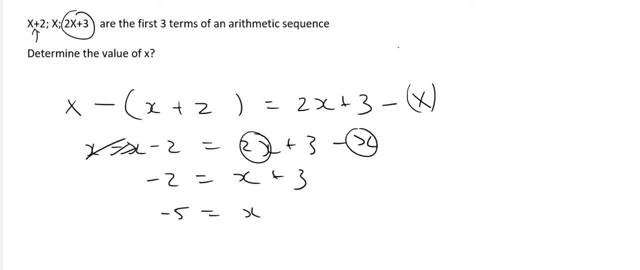 and then we can leave x on the right hand side and take that number over, and so x is minus 5. if you needed to know the original sequence, then you could fill x in, so the first term is minus 5 plus 2, and then you could fill x in, so the first term is minus 5 plus 2. 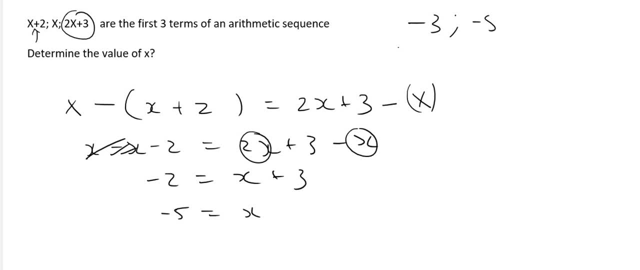 and then you could fill x in. so the first term is minus 5 plus 2, which is minus 3. the second term is just x, that's minus 5, and the third term is 2 times minus 5 plus 3, and that's going to give you minus 7. 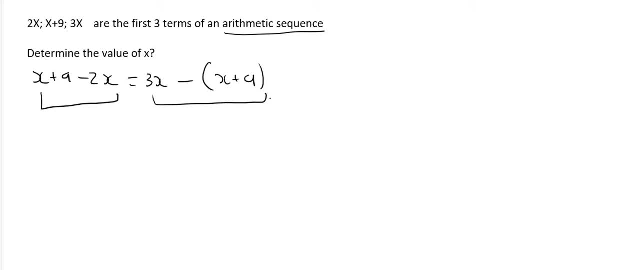 fact that the differences in an arithmetic pattern have to stay the same, So we can form a relationship like that. So what we have is x plus 9 minus 2x equals to 3x minus x minus 9.. And now it's just a matter of solving for x. So on the left hand side and on the right hand side. 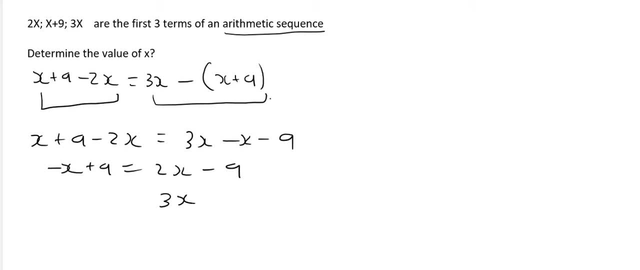 we have that, Then I'm going to take all the x's to the right and then bring all the numbers over, And so what we find is that x is equal to 6.. So if you then wanted to carry on with the sequence, 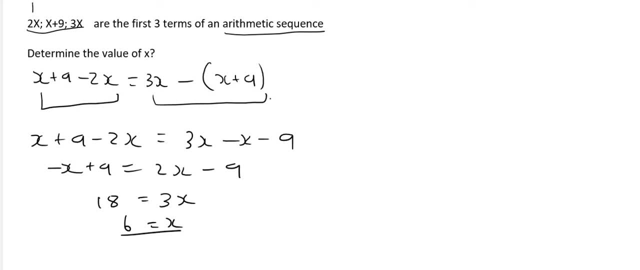 if there were other questions, you could fill in the actual values. So 2 times 6 is the term on the left. So if you wanted to carry on with the sequence, you could fill in: the actual is 12,, 6 plus 9 is 15, and 3 times 6 is 18.. And so this is the original pattern, and then you could. 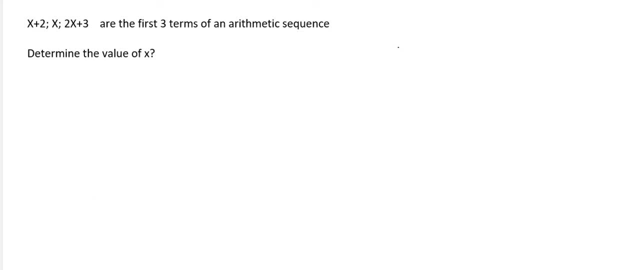 use that. if there were other questions, Here's another one that we can practice. So we know that when it's arithmetic we can take the second term minus the first term. and remember, when you're minusing something with two terms, or two or more, you want to use a bracket, Then you're. 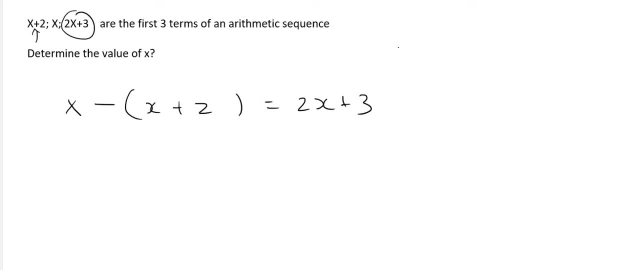 going to make that equal to 2x plus 3, which is this term over here, minus the middle term, which is x, and you can put that in a bracket if you want, but there it's not going to make much of a. 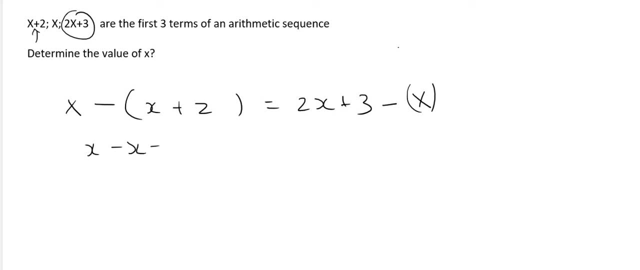 difference. Now what we do is we just solve so it becomes x minus x minus 2 equals to 2x plus 3 minus x. These x's cancel and so minus 2 is equal to x plus 3, because this 2x minus that x is just. 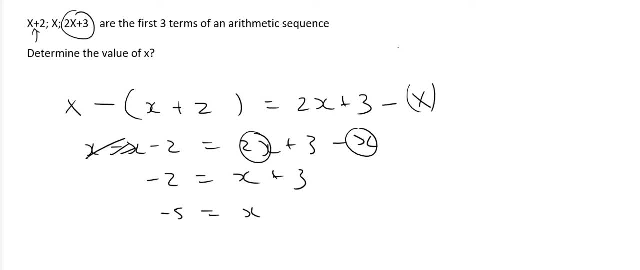 x, and then we can leave x on the right-hand side and take that number over, and so x is minus 5.. If you needed to know the original sequence, then you could fill x in. so the first term is minus 5, and then you could fill in the second term, and then you could fill in the second term, and 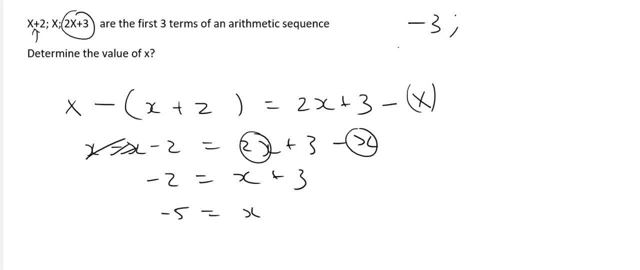 then you could fill in the third term, and then you could fill in the fourth term, and then you could 5 plus 2, which is minus 3.. The second term is just x, so that's minus 5, and the third term. 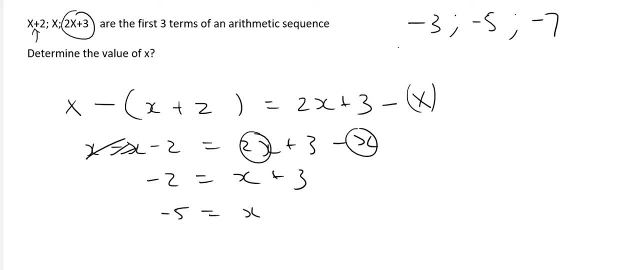 is 2 times minus 5 plus 3, and that's going to give you minus 7..